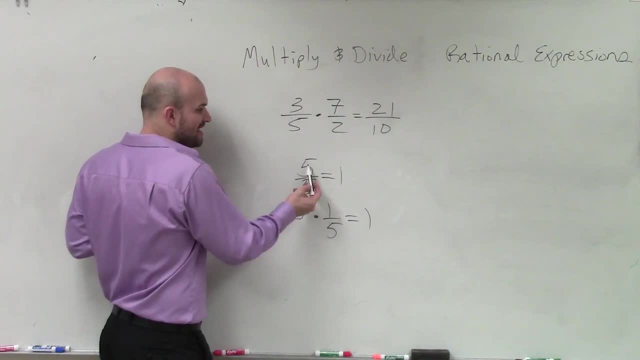 I'm getting the exact same solution: 5 divided by 5.. 5 divides into 5 one time, 5 times the reciprocal of 1 over 5, because you can write 5 as 5 over 1.. When you multiply a number by its reciprocal, that 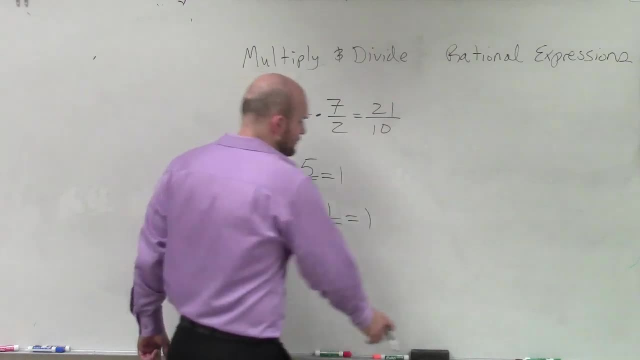 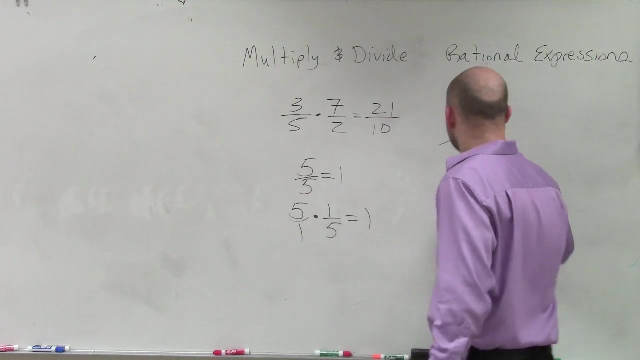 equals 1 as well, So there's a couple different ways to look at this. For instance, if I had 1 half divided by 3, fourths, a lot of students. if we look at it in this way, you might say: 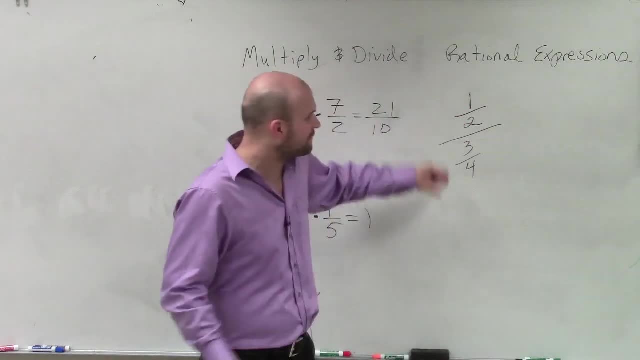 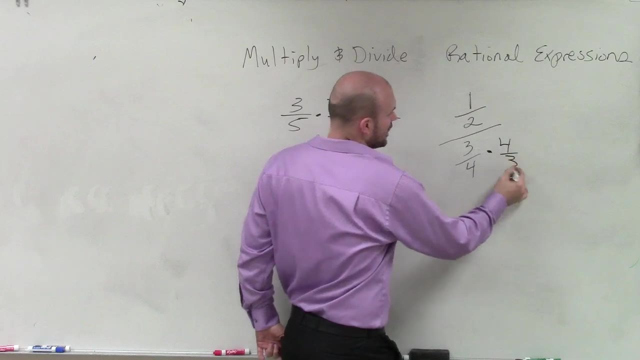 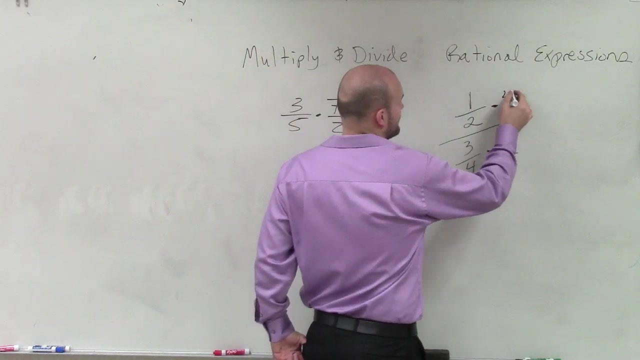 I don't remember what to do. Well, when you have a fraction in the numerator and denominator, a lot of times we call these complex fractions. if I multiply by my reciprocal of 4 thirds, I know that that's going to produce 1.. But remember, by producing equivalent fractions. 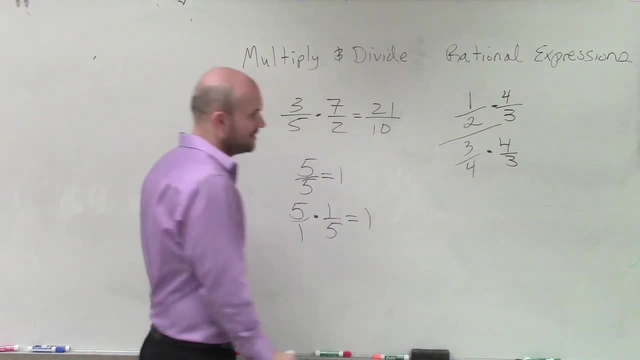 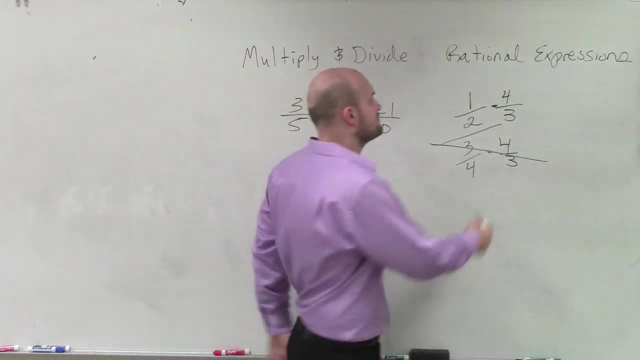 whatever we multiply in the numerator, we have to multiply by the denominator, So any number by its reciprocal, it multiplies to 1.. But then I'm just left with 1 divided by 2 times 4 thirds. So what's important about that is if I have 1 half divided by 3 fourths. 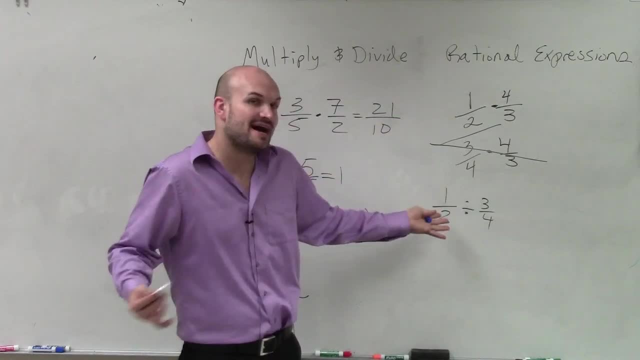 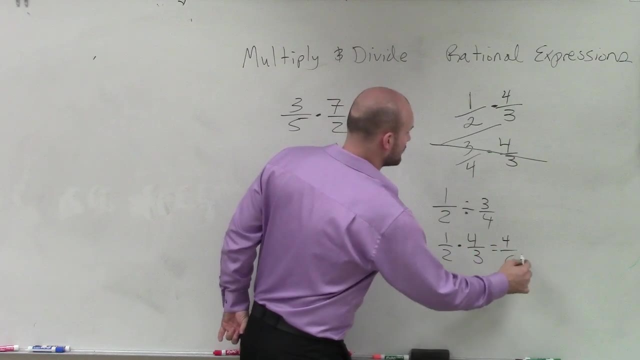 I just have to look at it as the same thing as 1 half over 3 fourths And, to finalize this problem, just make the reciprocal and then multiply, So in this case we'll have 4 over 6, which, remember, we can always reduce down to 3 halves, And reducing is going to become 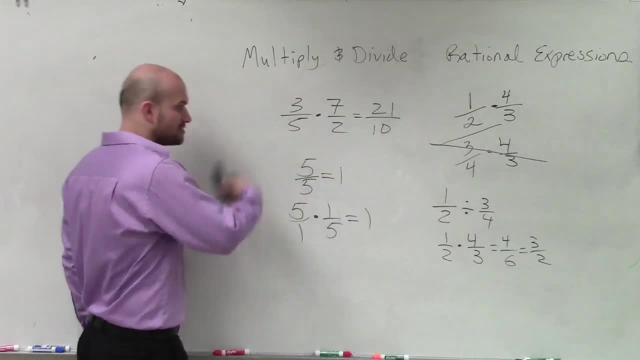 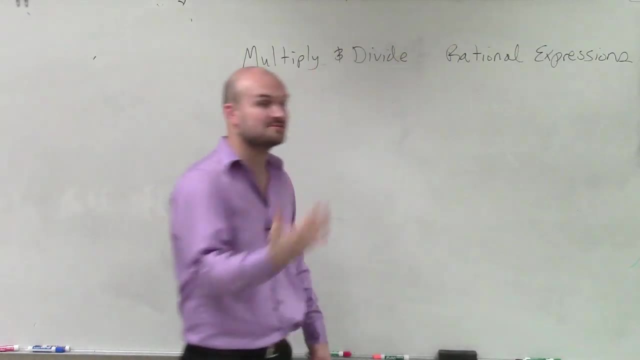 very, very important in this course. So that's at least the process of why, when we divide, we multiply by the reciprocal, And when we multiply we just multiply across. Now, when rational expressions, there's a couple things that become very important. 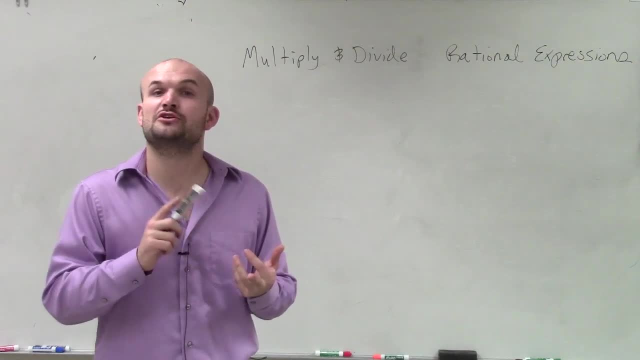 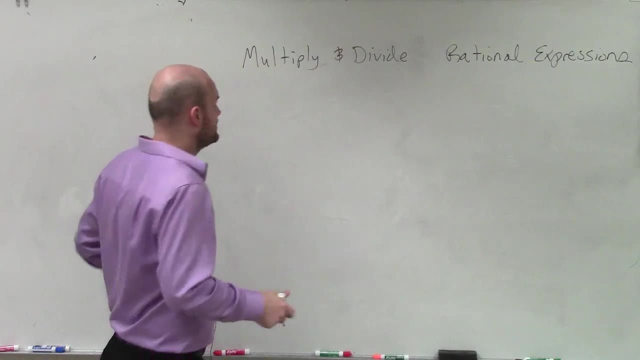 One is simplifying and reducing, And the other one is make sure you can apply your multiplication by using FOIL and so forth, And also looking to factoring to simplify this. Now, for instance, let's say I had an equation here of x. 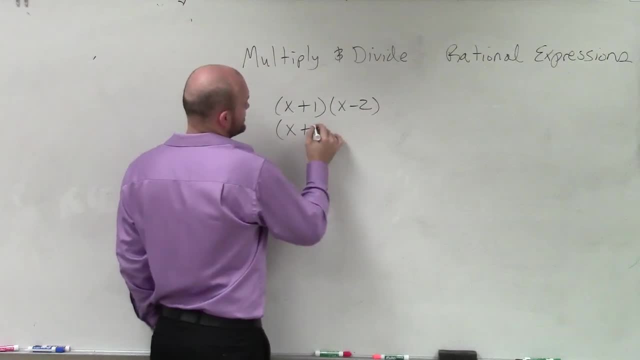 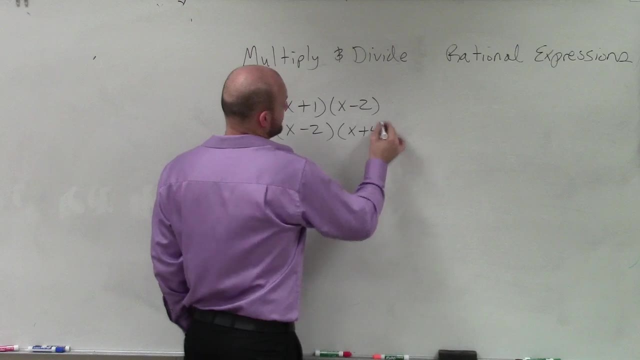 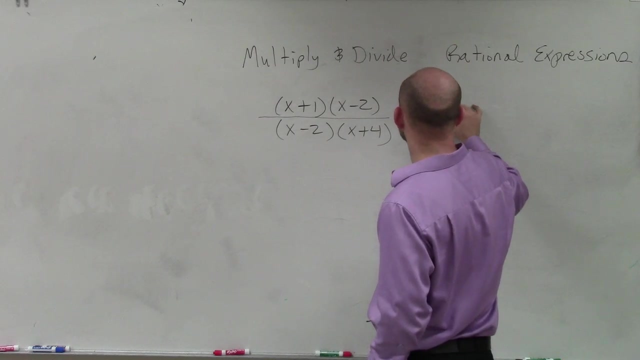 plus 1 times x minus 2, over x plus x minus 2 times x plus 4 times. And then let's again do x plus 4 times 5 divided by x plus 1.. Now you might be crazy looking at this problem and saying: 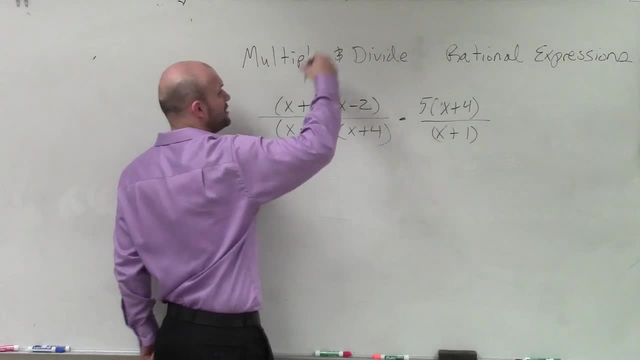 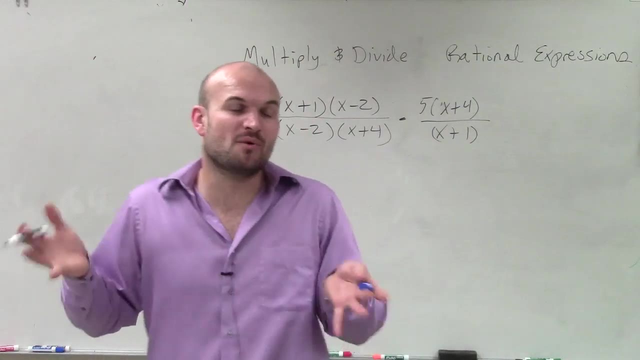 oh Well, let me just multiply all these out. So that means you're going to multiply a binomial times, a binomial times, a monomial times, another binomial. Then you have to multiply all three of these binomials again. So we're multiplying. 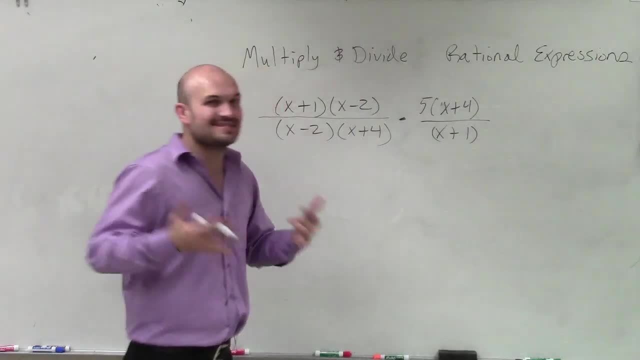 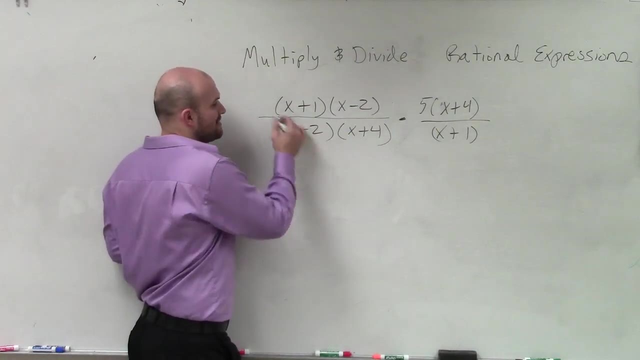 The best thing I tell my students to look for is look for ways to simplify this. Look for ways that you can divide out terms equal to 1.. And what's nice about this? you can see my x divided by 2 divides out my x divided by 2.. 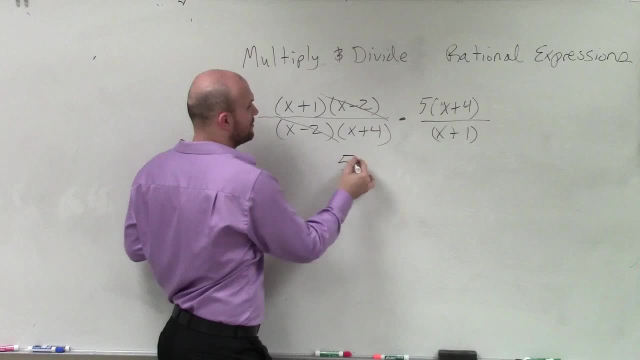 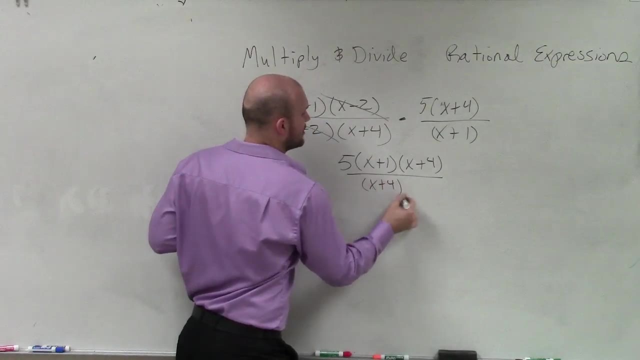 Then, when I multiply this across, without multiplying my binomials, I'm left with 5 times x plus 1 times x plus 4, divided by x plus 4 times x plus 1.. So rather than applying FOIL to simplify that out, 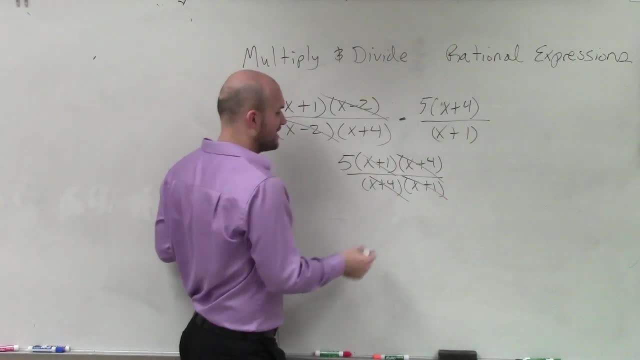 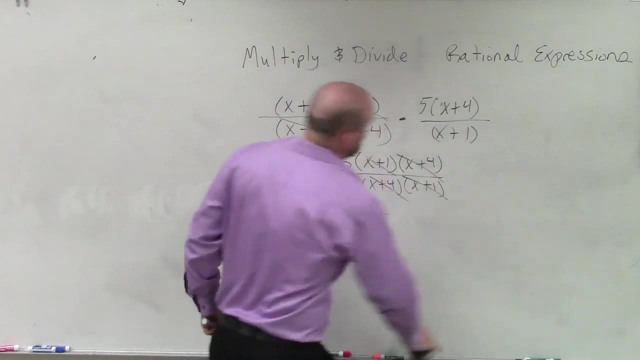 I can see that the x plus 1's divide out and the x plus 4's divide out to 1, just leaving me with a simplified answer of 5.. So always try to look for those opportunities, And those are going to happen. a lot by factoring. 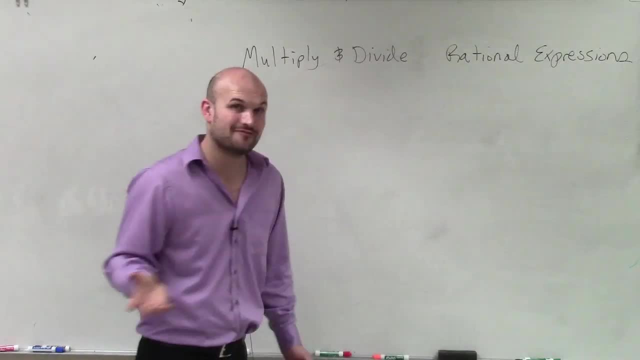 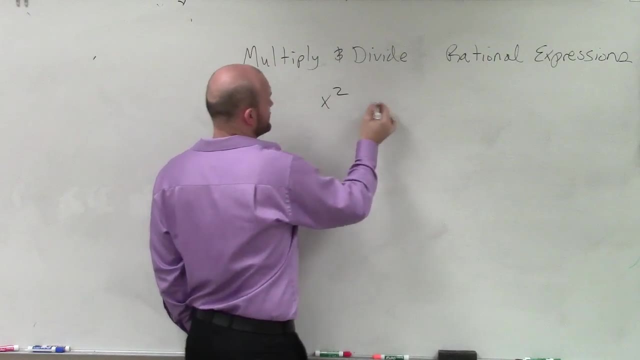 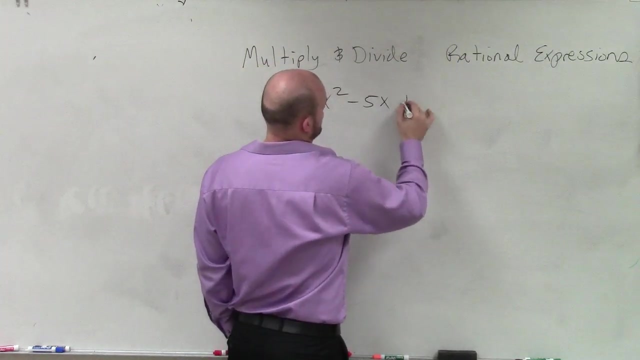 I'm just going to give out a problem. Let me see if I can figure, if I can get one in here, If I can multiply one out. So let's do x squared minus 5x plus 6.. All right, And now let's do divided by: 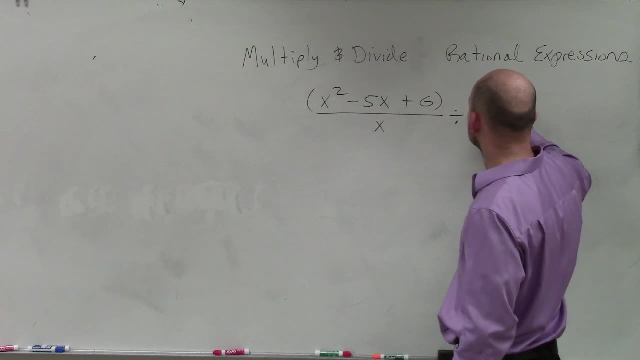 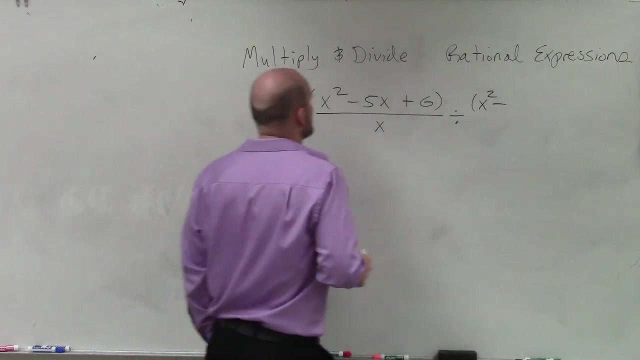 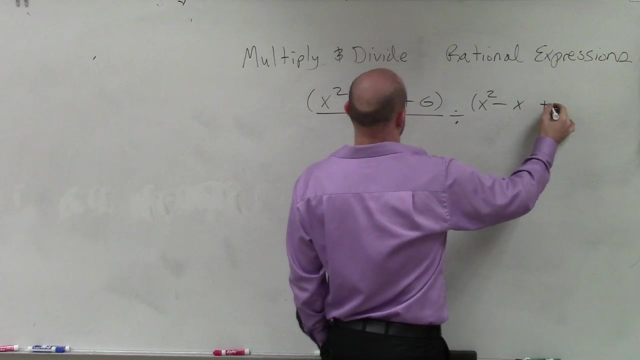 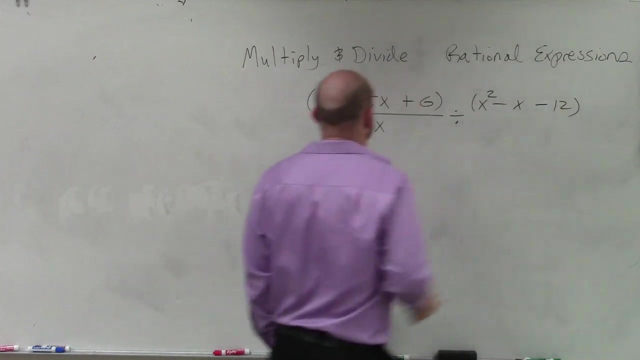 Divided by x squared minus x plus 12.. No minus 12.. No minus 12, yeah, OK, And I don't know. Let's do this over x again, OK, So if I was going to do this again, we know that division. 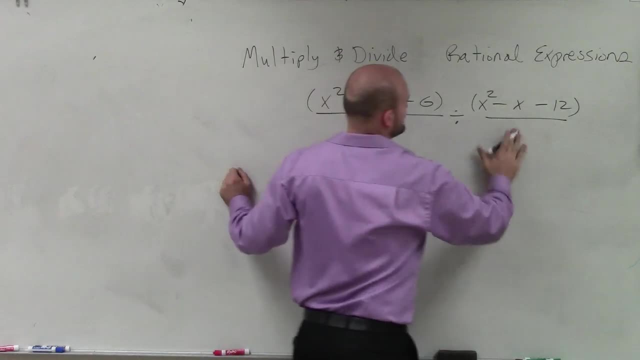 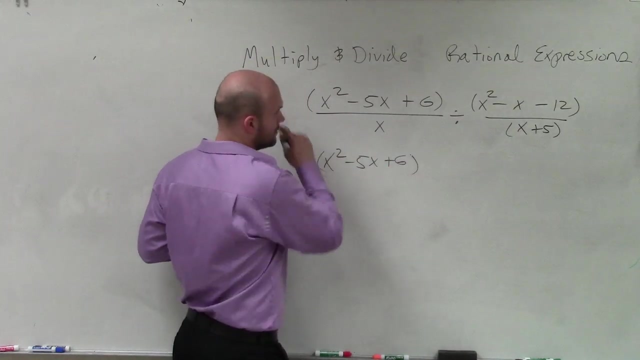 We can rewrite this, So it's going to be x squared Actually. let's make this a little more difficult. Let's do x plus 5.. OK, So I have x squared minus 5x plus 6 divided by x. 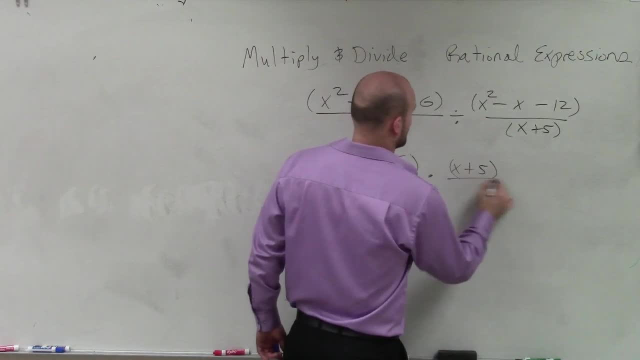 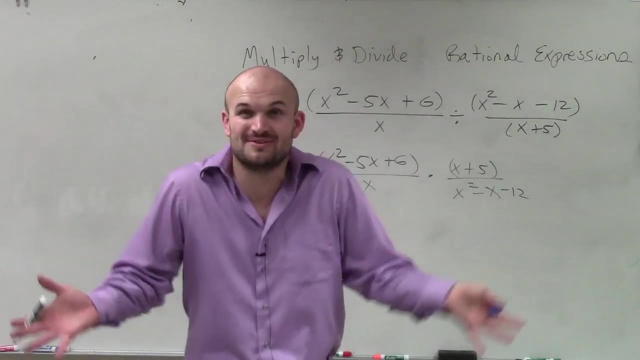 Now times the reciprocal of that, which is x plus 5, over x squared minus x minus 12.. Now again you look at this. you say, ah, I wish I could cancel things out like the last problem, But you can't.